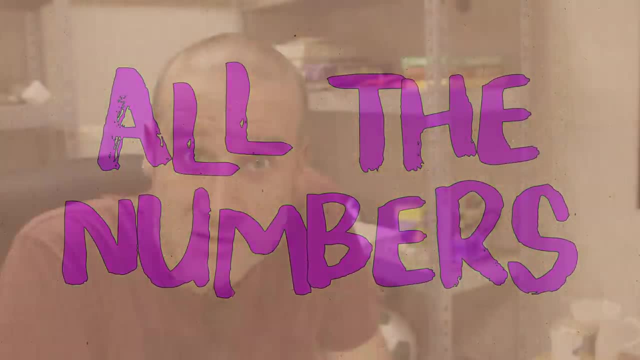 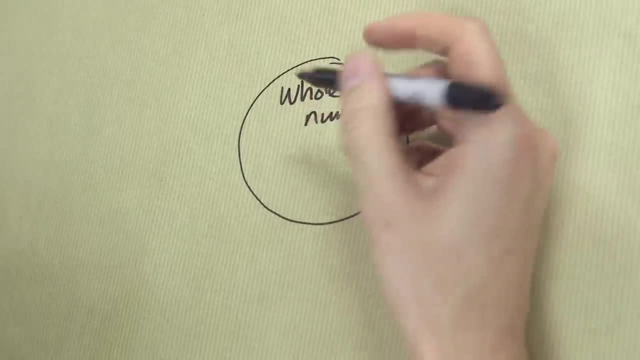 We're gonna do all the numbers On Numberphile. we've done a lot of the numbers, some would say, but we haven't done all the numbers. Originally we did the whole numbers and these are the classics. I guess we've done 11, that was an early one. We've done 3, 4,, 3, 5,, 17, right. 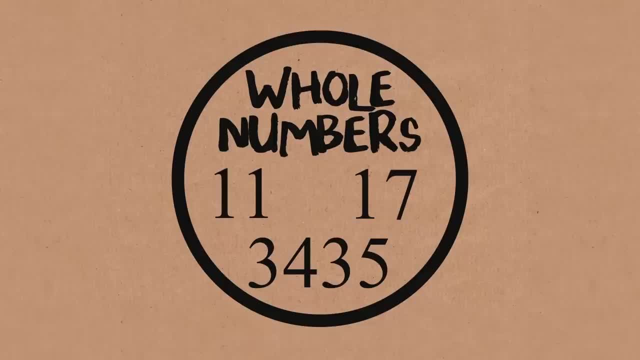 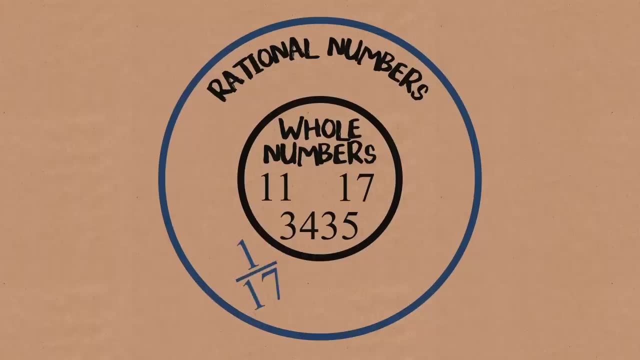 All the whole numbers sit in here. But then there are other types of numbers If we go one step out: the rational numbers, the ones that are ratios, these are, you know, you get a 17th, you get- I don't know things- over a 12,. you get all sorts of. 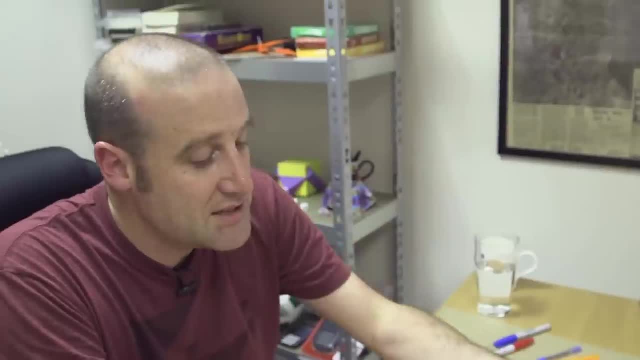 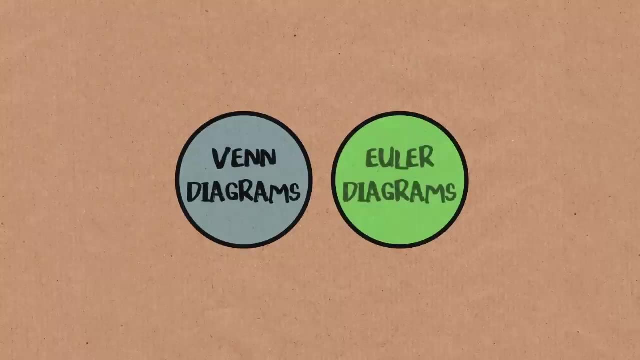 So now you've got all the rational numbers. We've gone beyond that, though, and the rationals technically include the whole numbers. they're a subset, but I'm doing this as what people call Venn diagram, which is wrong. It's an Euler diagram, because I'm not showing every single possible combination. 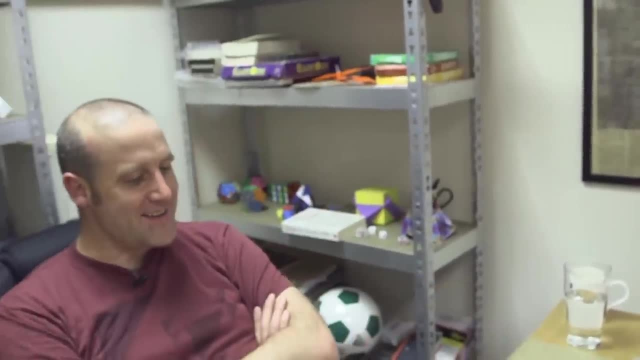 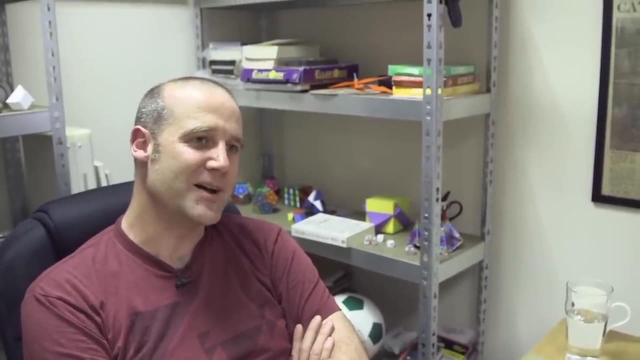 And negative numbers, whole numbers. You know I put in a 12th because I thought I was being hilarious and then I immediately thought I wasn't gonna put negatives on this diagram. So I regret that for two reasons: opening the negative can and the expression on your face. 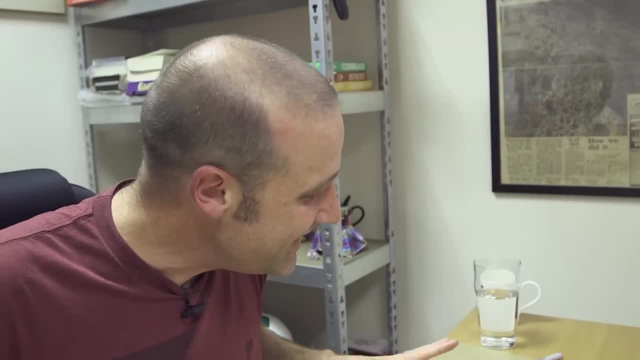 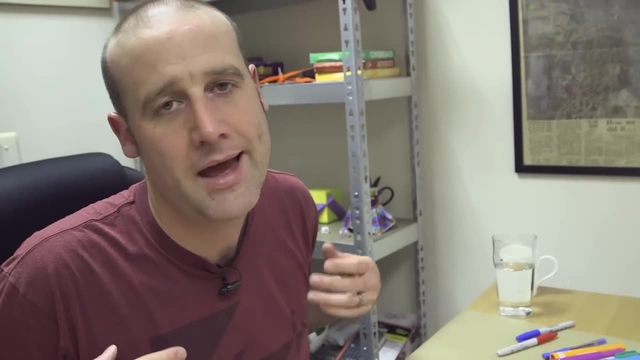 So I'm gonna make a. Make that a plus. there we are. In fact, this whole sheet of paper is just gonna be the reals, positive reals, You know what it works for? negative reals. What am I saying? Have the negatives, it's fine. 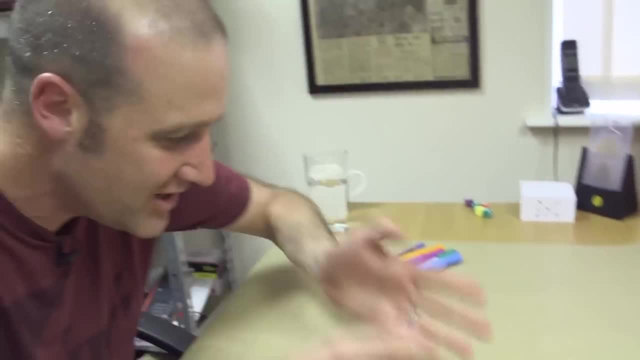 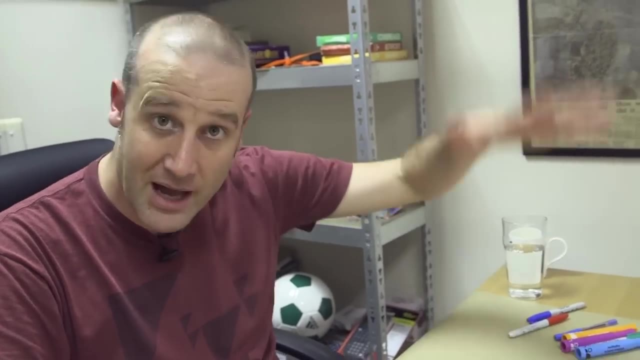 But the sheet are all the reals and inside here I've put whole numbers and then I've put rational numbers. If you can obviously get complex numbers coming up, we're not gonna do that, we're gonna stay down here. 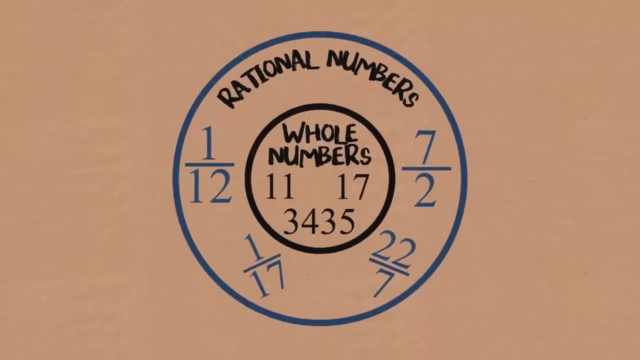 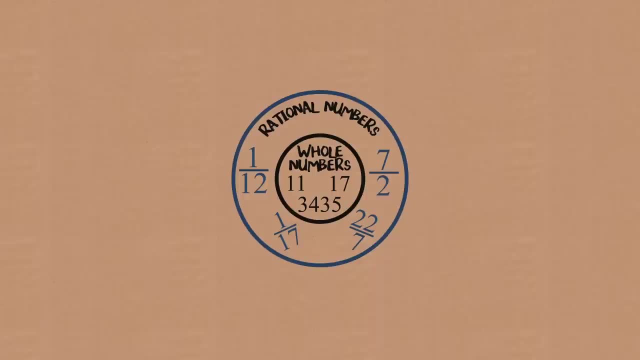 And I'm gonna basically work our way out until we get a greater distance out than number 5 has ever gone before. Right, we're going for the new Numberphile record. How far out into the weird reals can we go? But we've done rational. Next one up are the constructibles, and these often aren't mentioned. 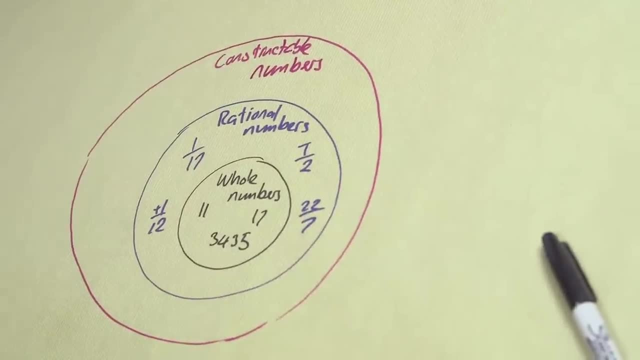 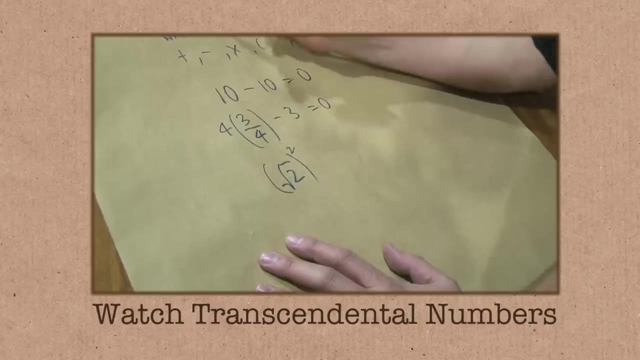 You don't have to add this in as a category, but I quite like constructibles. More importantly, what people tend to go for? the next one out are the algebraic. Okay, so Simon did a fantastic video about algebraic numbers and when you go outside, 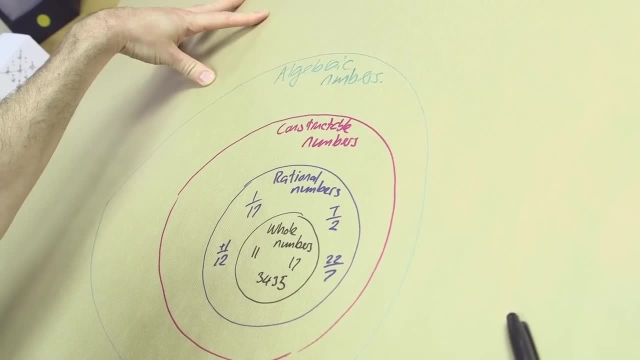 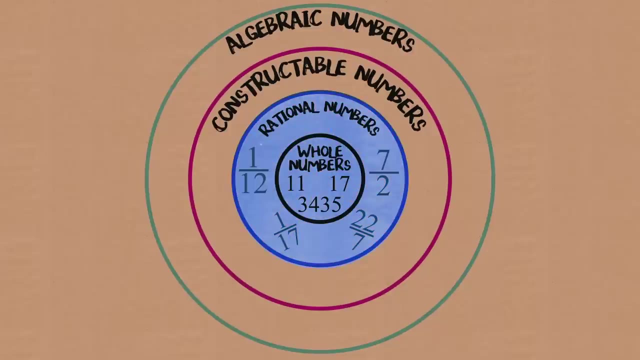 Transcendental numbers. I mean this number is really, really important and no one knew, And so a lot of the number categories refer to in or out Of these different sets. So rational numbers are everything inside the blue line. 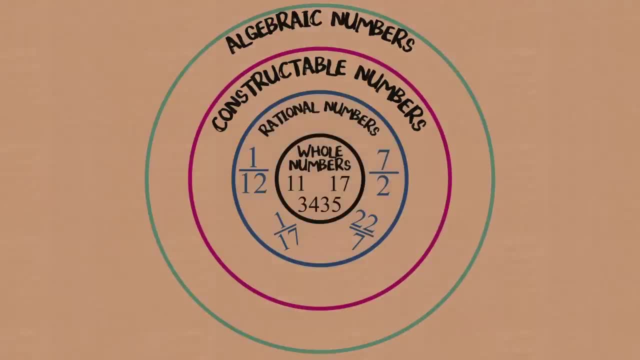 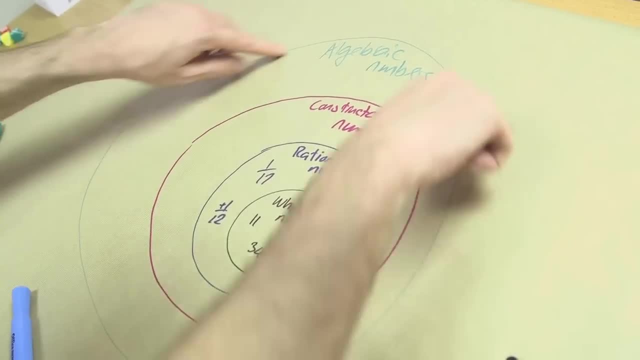 Irrational numbers are everything outside the blue line. You've got constructible numbers or anything inside the purple line. Unconstructible numbers are outside this and this light blue line out here. algebraic numbers are everything inside there and Transcendental numbers are everything outside of there. 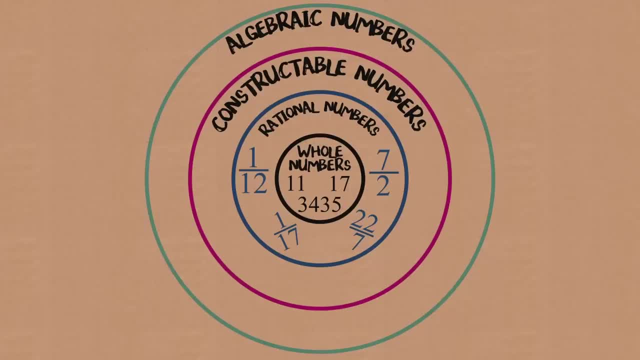 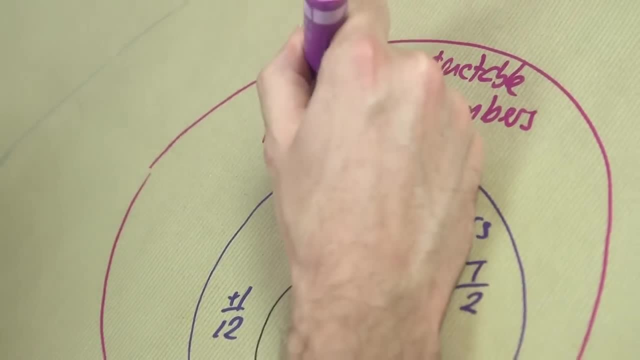 And so constructible numbers are things that you can construct with a pencil and a compass and a ruler. So phi, you can do that. the golden ratio, because you can do roots Five, so you can get phi, You can do root two. that lives in here. 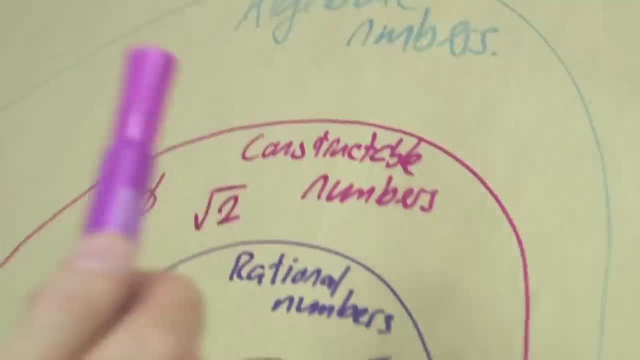 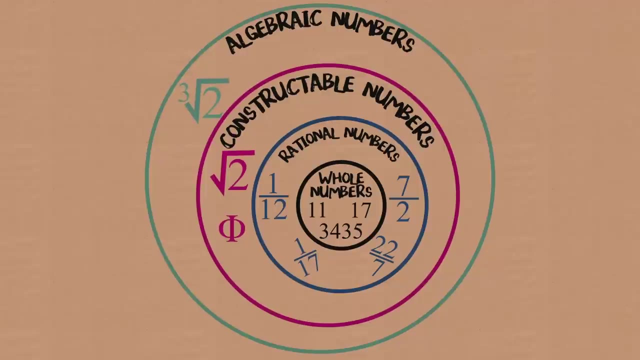 It's kind of fun. Algebraic numbers are the solution to an algebraic equation. If it's a square root or lower, you can put it in constructible, You can draw it. If it's higher than that, you can't. So the cube root of two is an algebraic number. 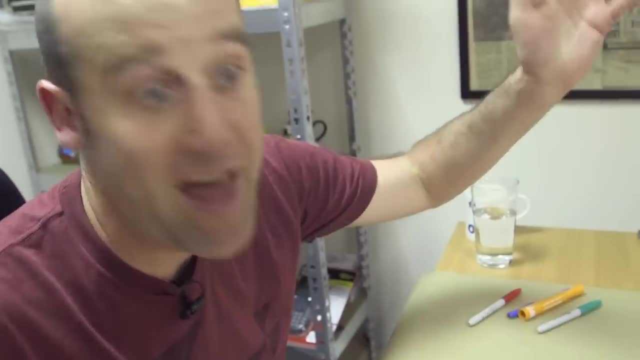 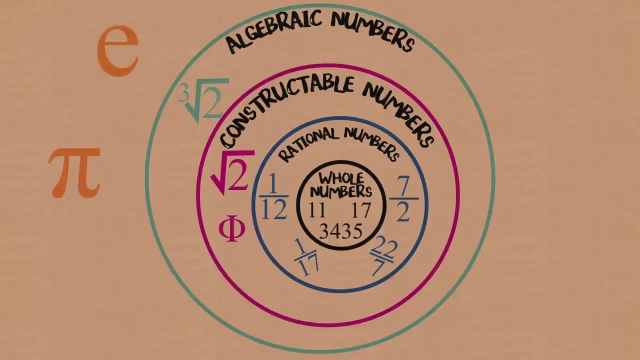 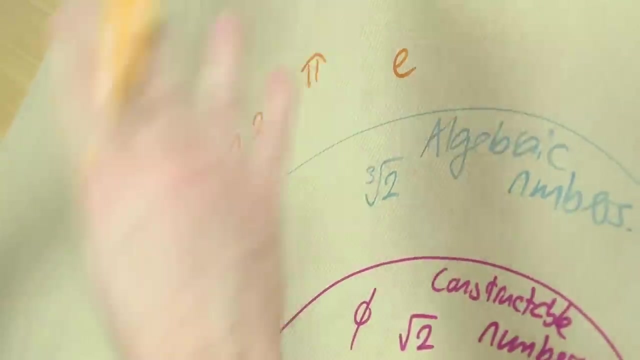 And then outside algebraic you've got beyond that, right? So you've got things like pi. Pi lives out here. Pi is transcendental, E is transcendental, The natural log of two, that's out there. Things that aren't a nice neat solution to an algebraic equation, right, They're out there, right. 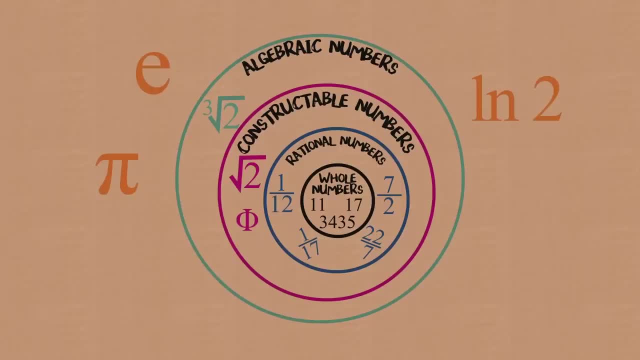 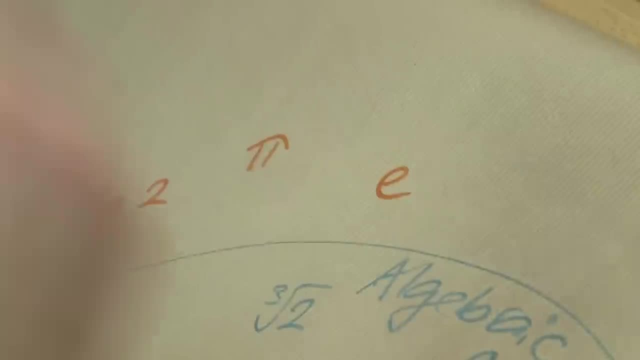 This is how people tend to categorize all the numbers, And this is the fringe of kind of what we understand in mathematics and what we've done on numberphile. So E was the first number that was proven to be transcendental, and so that was proven in 1873. 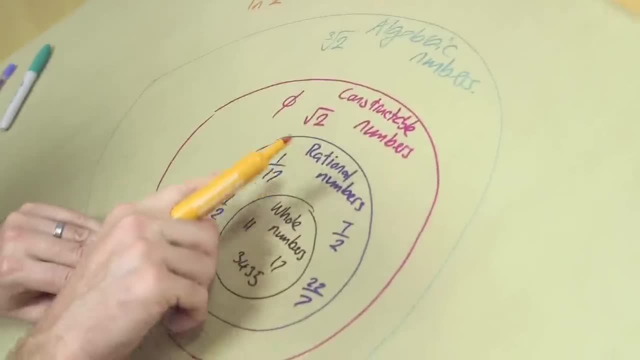 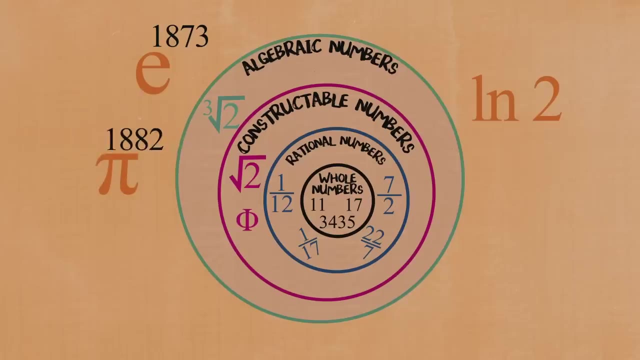 So reasonably recent, given that some of these are thousands of years old. We knew it existed, but we didn't know where it went. Pi- we didn't know where that went. Pi was proven to be out here in 1882.. 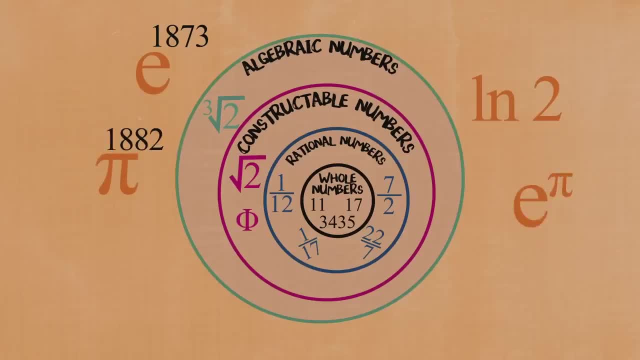 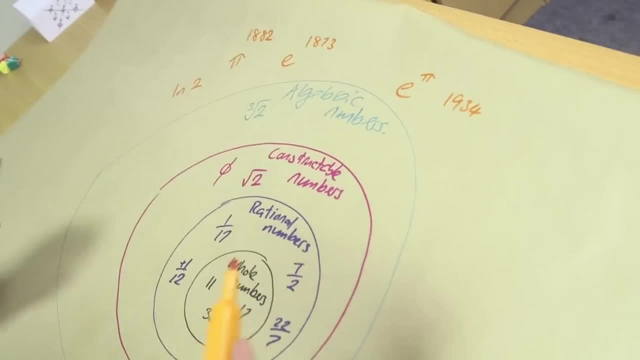 So E to the power of pi was proven to be out here in only 1934. So that was a more recent one. we managed to prove is out there And there are loads which we don't know. Pi to the E we don't know. 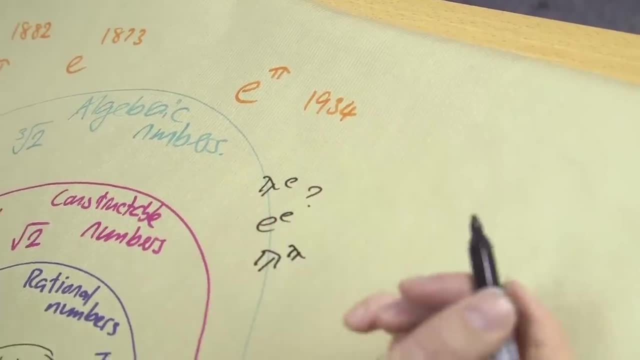 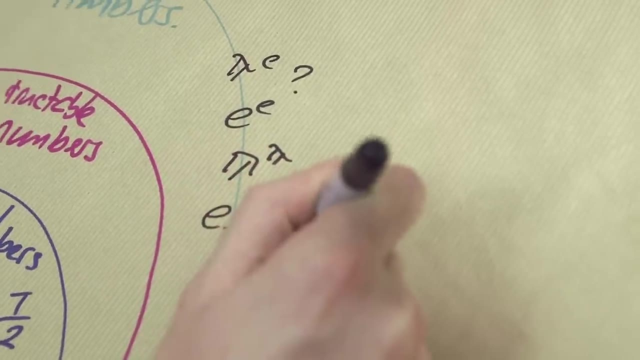 E to the E. we don't know. Pi to the pi. we don't know. right, These are all on the cusp. We know that one of E times pi, or E plus pi, one or more of those are transcendental. 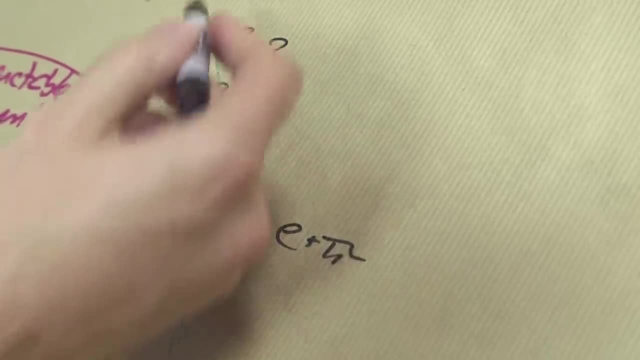 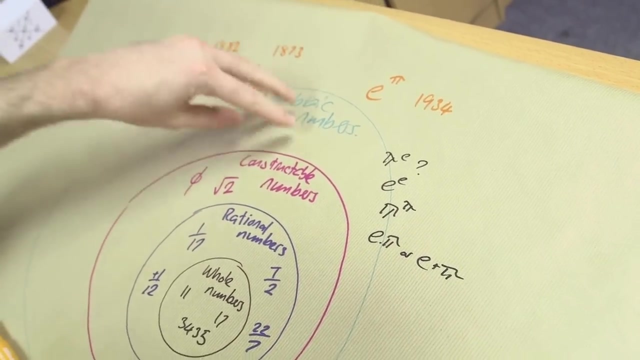 We don't know which or both right, But we know at least one of them is. Most numbers that we know are algebraic sit around here and we don't know if they're definitely transcendental or if they're still algebraic. For the most part we haven't got a clue right. If you look at the entry for transcendental numbers on Wikipedia or Math World, there's a list. Here's the only ones we know, and that's it right. Some of our favorite big old numbers: 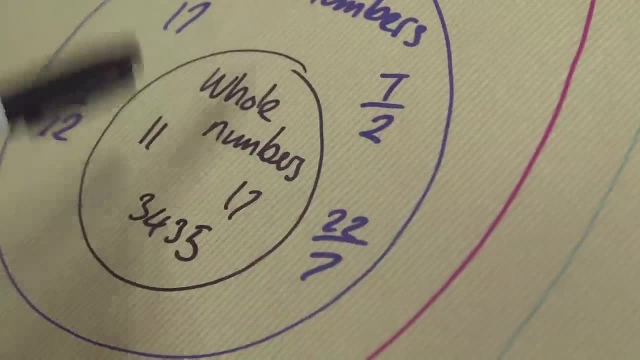 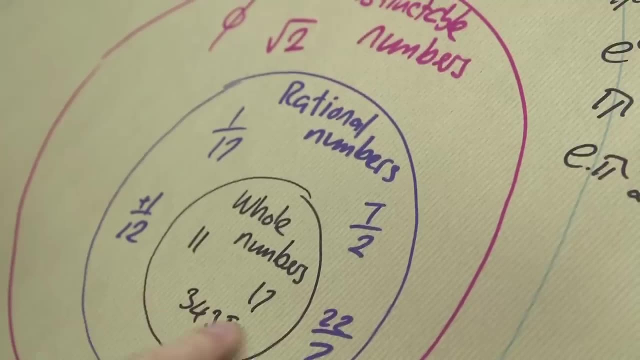 Graham's number in here. It's in here, right? Whole numbers, doesn't matter how big it is, it's in there. There are infinitely many whole numbers, but there are also infinitely many rational numbers. Same infinity. There are infinitely many constructible numbers. 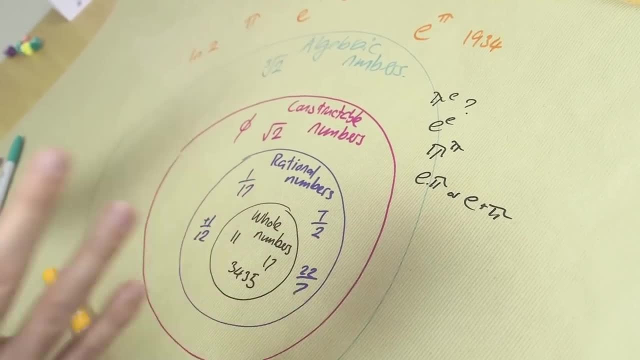 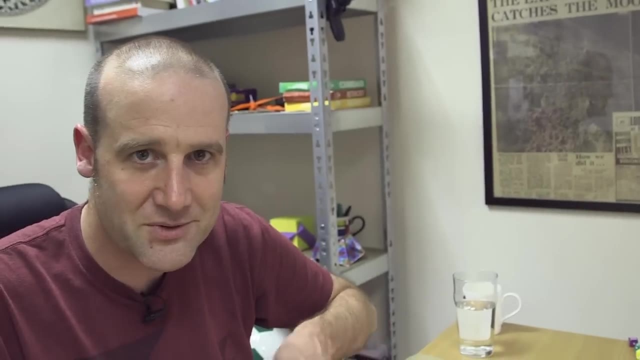 infinitely many algebraic numbers, but all countable infinity is the smallest infinity possible. the many of these numbers in here And there is one more circuit out. You know what Should we chuck? on the last one I can add another loop and it cleans up all of these. 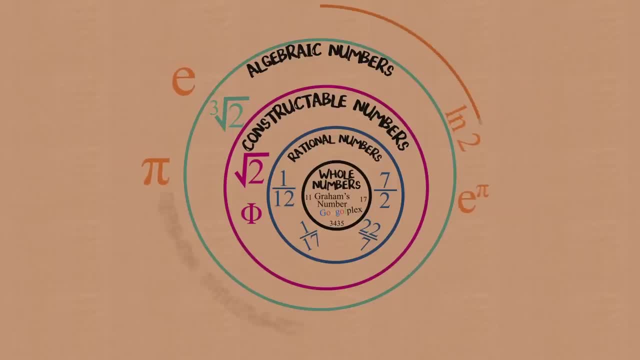 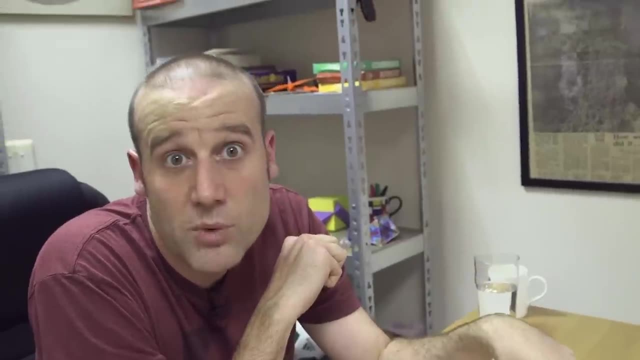 and it puts them all in a neat bow. This is the collection of computable numbers. Computable numbers. what does that mean? It just means we can compute them. So we can compute E, We can compute pi. right, It's not the solution to a nice equation. 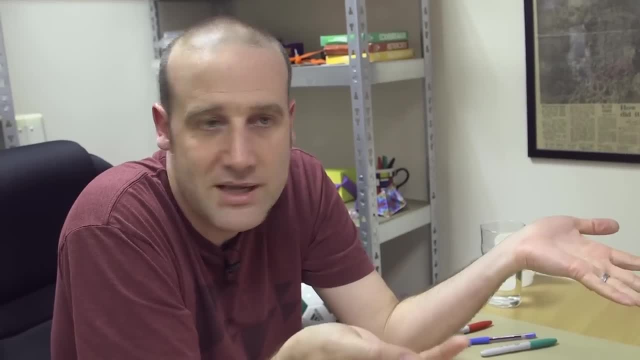 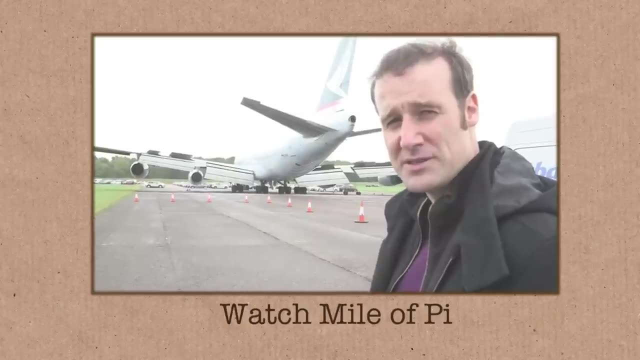 but I can write down a system by which you will get the decimal places right, And so we do this. We print them out on a very long bit of paper, roll them out on a runway. It's hilarious, right? We're here on a runway because, for some reason, Brady has printed out. 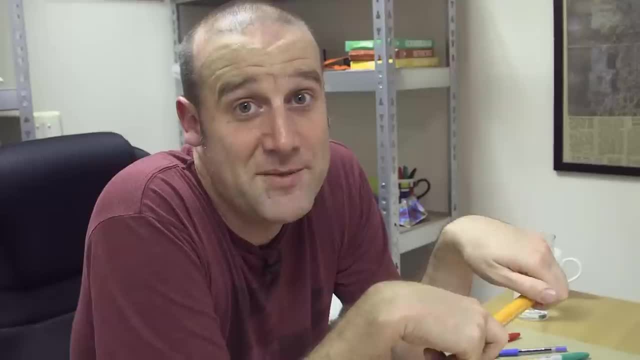 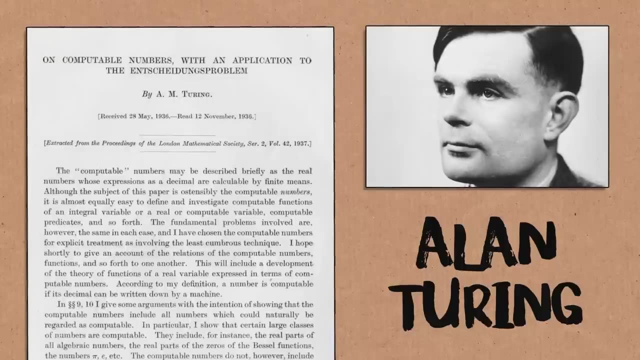 the first one million digits of pi. So this came down to Alan Turing in 1936, and everyone remembers that Turing invented the computable numbers, The Turing machine, And that was in his paper on computable numbers. He was looking at if you can compute all numbers. 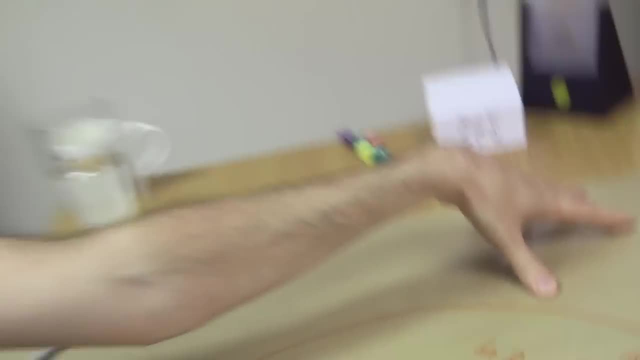 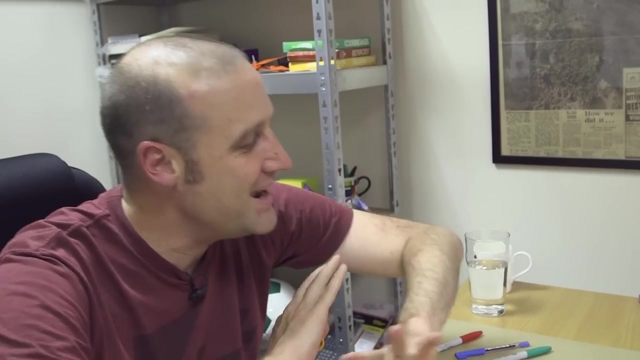 and he showed. there are numbers that exist out here, but we just don't know what they are. I call them the dark numbers, right, All these numbers that we know they exist, Turing showed us, but they're so hard to grasp. 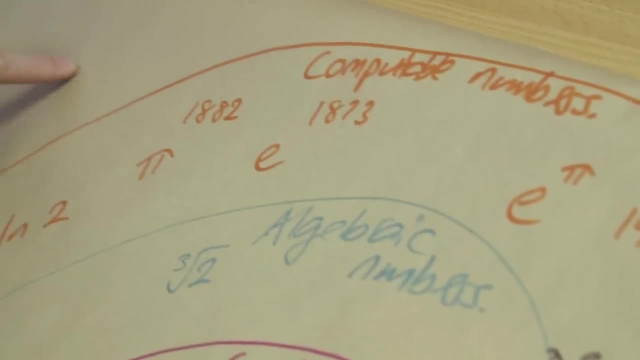 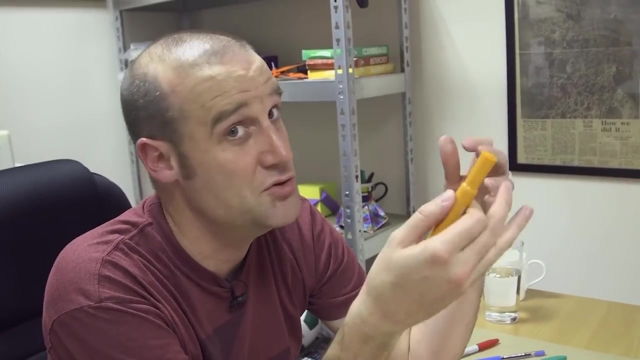 And occasionally we see them, but not often. Well, hang on, why isn't pi out here? We can compute pi. Well, it takes forever. Like I could write down an infinite series which gives you pi, And I can give you the rules for writing out the infinite series. 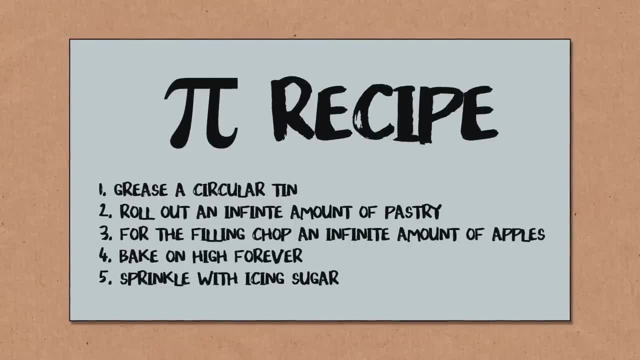 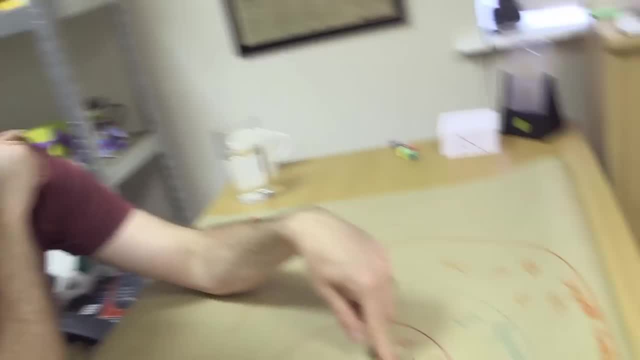 and I could write them on a postcard or some finite amount of space and go: here are the rules for calculating pi. You're going to have to do them forever, but the rules are finite. So for everything else in here, I can write a description of how to get all the digits. 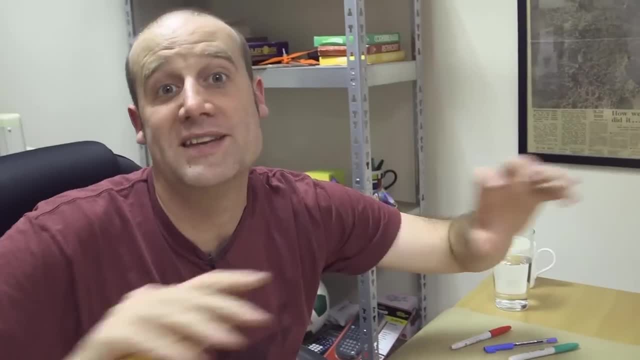 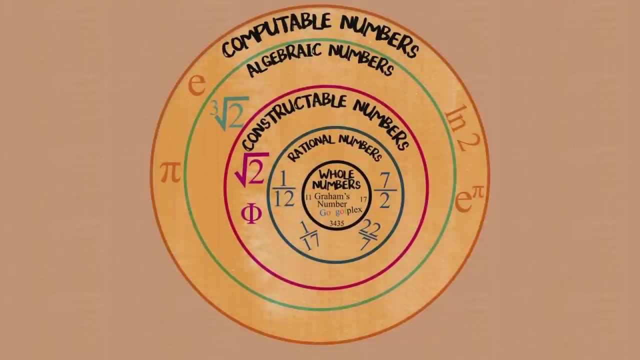 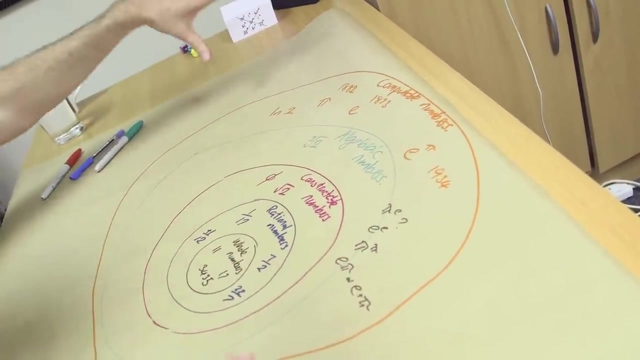 Out here. they're only definable by writing out all the digits, And that's actually most numbers In here. this is the countable infinity land. right, There's infinitely many of these, but the smallest- infinitely many Out here, is a bigger, infinitely many. 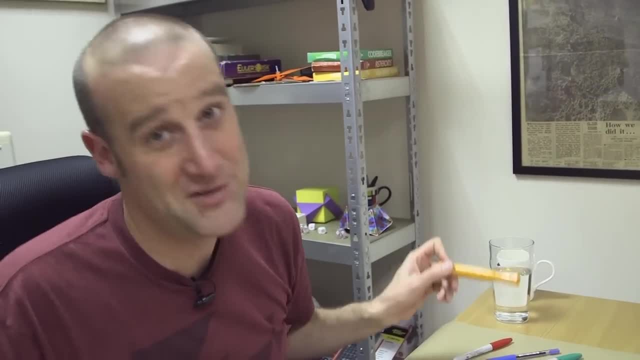 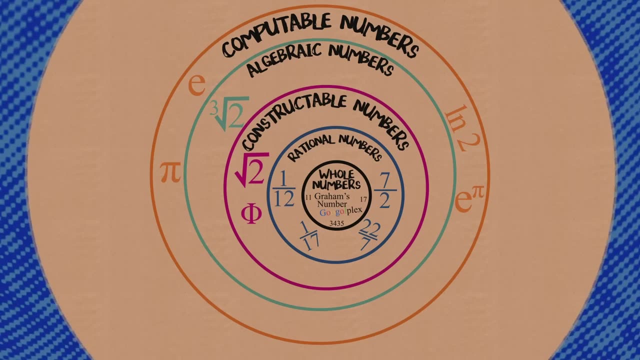 So the vast majority- for the strongest definition of vast majority you can come up with- of numbers are not computable. So we live in this nice little island of numbers that makes sense. And then outside is this vast, vast world of all the reals. 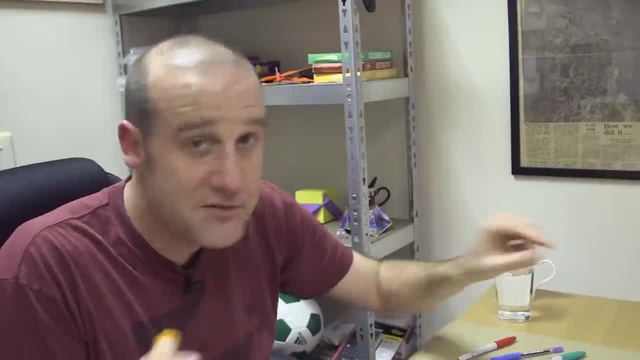 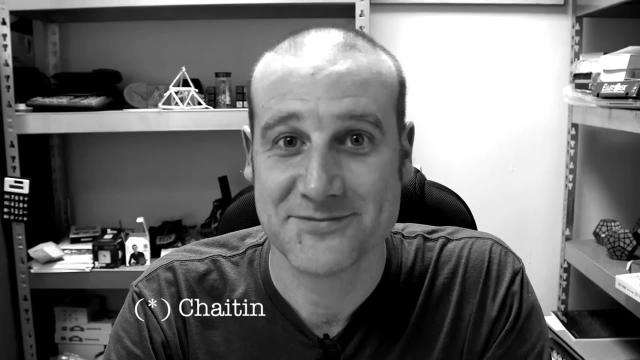 which are only definable by writing out their digits, And we've spotted a few. So there's one called the Chai-Lin constant. I'll have to double check. I got that right, Chaitan. Vaguely speaking, it's the probability. 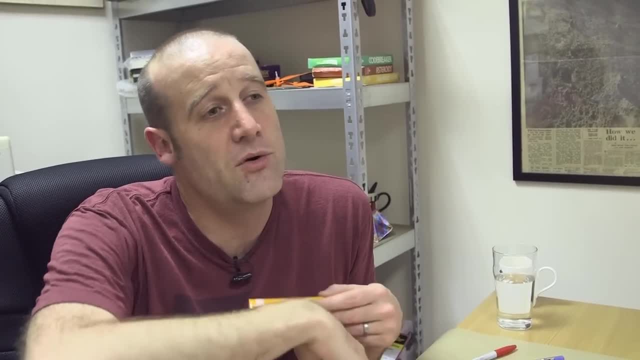 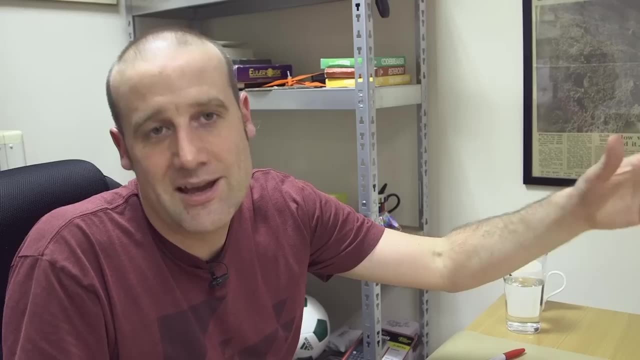 for a certain way of writing a computer program. if you generate a computer program at random, if it will run and come to a stop- And that probability, it's a naive way of describing it and it depends on how you write a program. 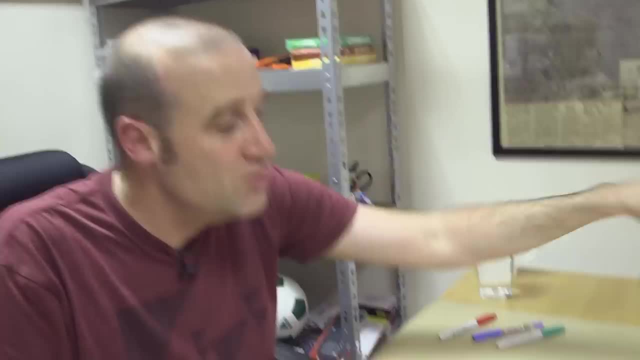 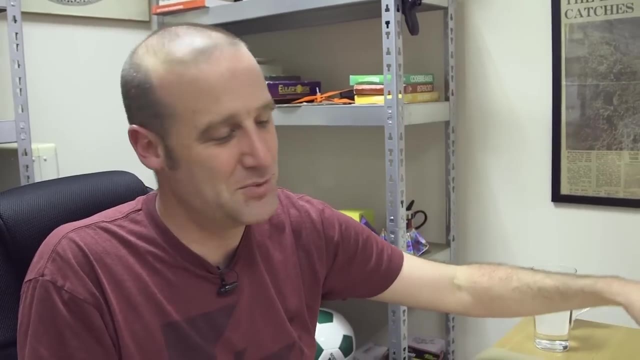 So in fact, there are lots of these constants, But we know they're all out here. The only way to get them is to work out every single digit individually. There's no equation, no algorithm that spits it out. It's an uncomputable number. And they're so mysterious and hard to understand, at the fringes of our comprehension of numbers. But they're out there And the scary thing is, most numbers are out there. How can we even know one of them? It feels like an unknowable, unknown. 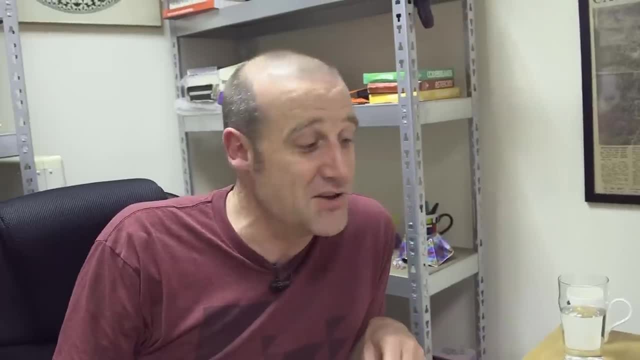 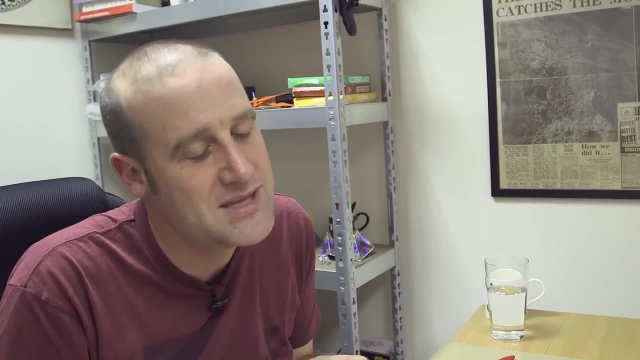 It is insane that we even know a couple of them, Because when I describe the numbers out here, I'm super hand-wavy because I don't understand them. I've read, I've tried, I read the paper. I'm like man, this is beyond me. 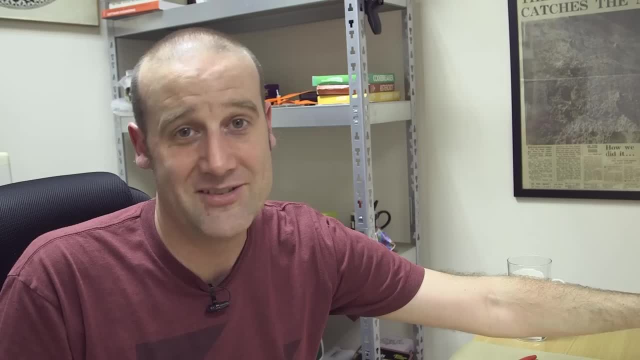 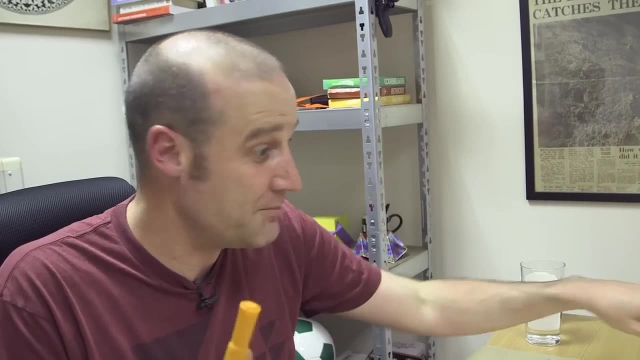 The maths. to try and grapple with the numbers out here is insane. But what's incredible is we have done it right. So if you look up uncomputable numbers, there are a few examples of ones out here, Although interestingly, 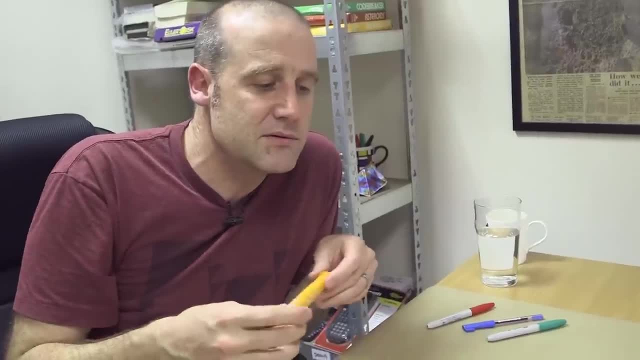 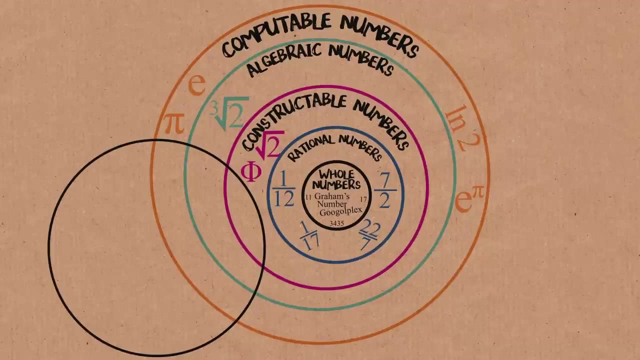 when you get these weird numbers. you can, you can- just you can- kind of make artificial ones. Okay, so I'm now going to kind of ruin my lovely neat diagram by putting on a whole new category. This is the category of what are called normal numbers. 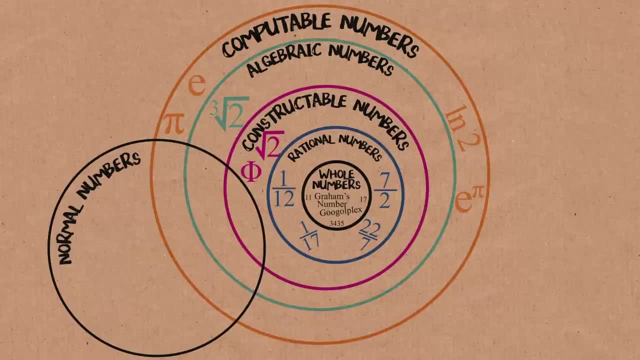 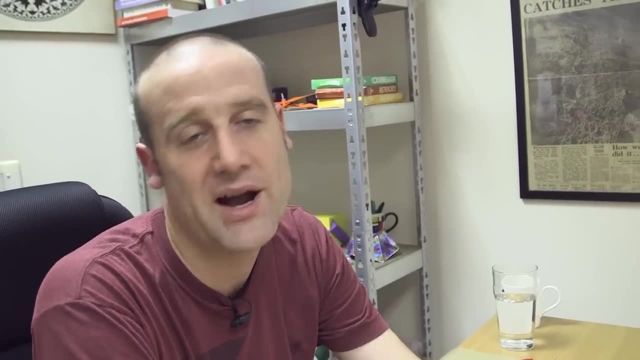 Which is a bit of a silly name. This means that every possible sub-grouping of digits is equally likely to be in there, And a lot of people say like, for example: pi Everyone goes, your phone number is somewhere in pi. 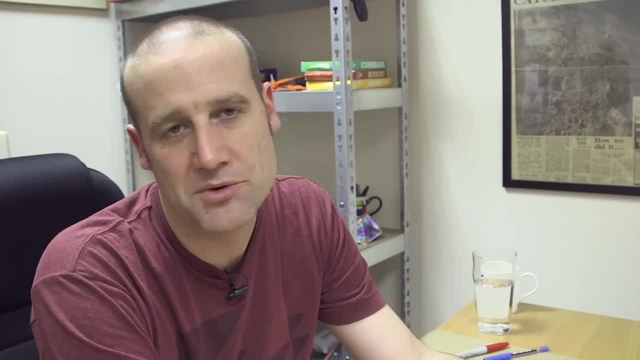 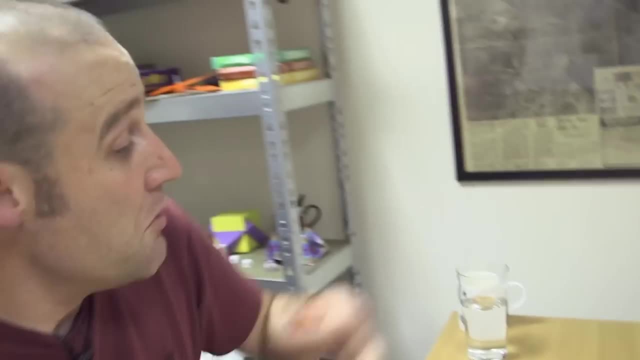 Your name is somewhere in pi. The complete works of William Shakespeare, if you turn it into digits, is somewhere in pi. We don't know that If we could move pi into here, Which we may yet do, We may yet do- It may be in here. 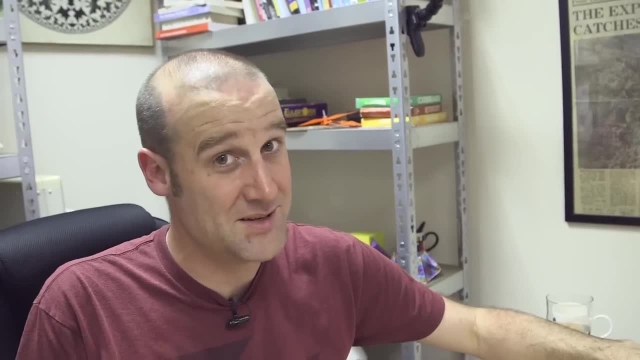 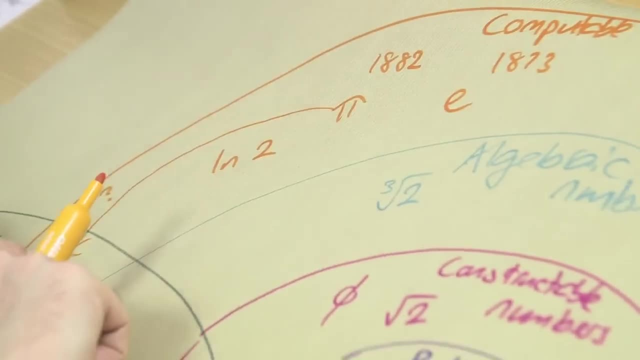 Everyone seems to think it is. All the digits we've checked imply it's in here, But we are not yet sure. We haven't managed to prove that. We don't know if pi is in here. We don't know if e is in here. 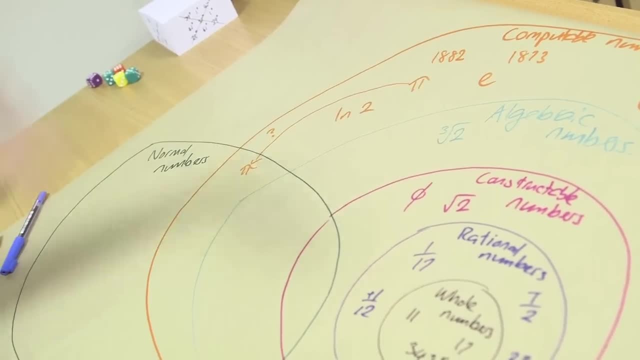 We don't know if root 2 is in here, Even though, for all of these, if you look through the digits you can find any string of digits you want. I found my name in all of them right, Because they've all got a lot of digits. 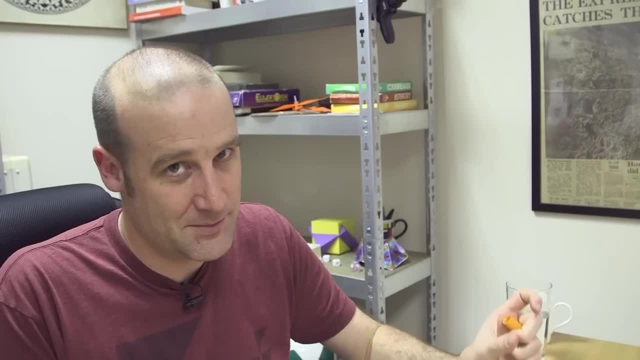 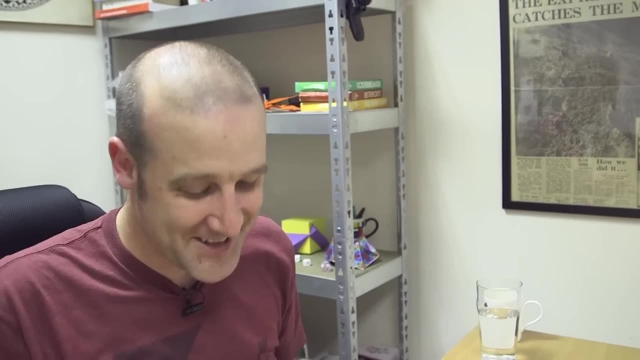 that are suitably random And you can find sub-strings in there, But we've not managed to prove any of those. are normal numbers. Would you like to see one number? we have managed to prove, So this: I love this number. 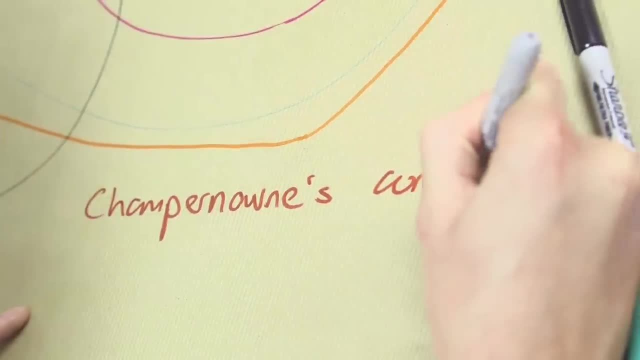 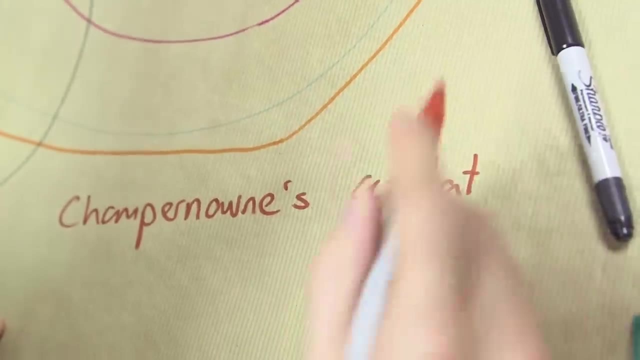 It's called temper nouns. constant Is normal. It's one of the few numbers we know is normal Constant. Constant, That's an N. Look at it, It's just climbing under the A. Oh yeah, So champ nouns constant. 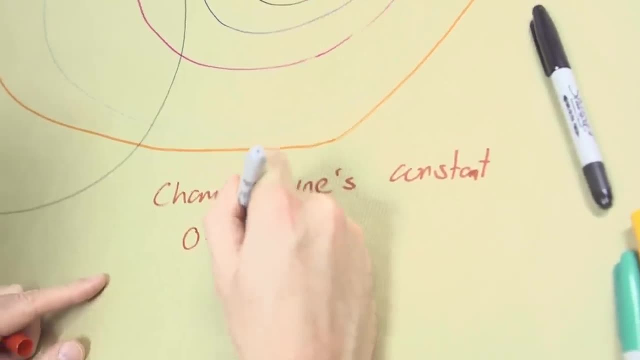 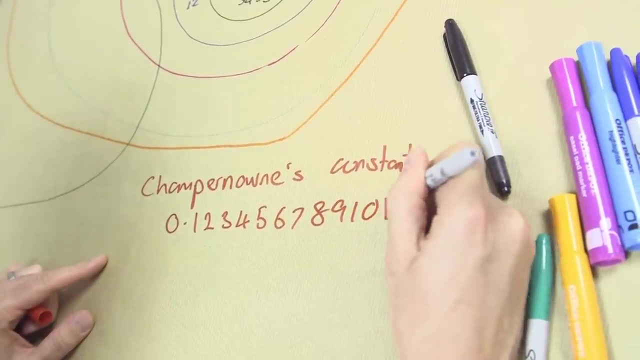 is one of the few numbers we know is normal And it goes 0.123.. I've memorized it: 4, 5, 6, 7,, 8, 9.. Well, 10, 1, 0,, 11,, 12,, 13.. 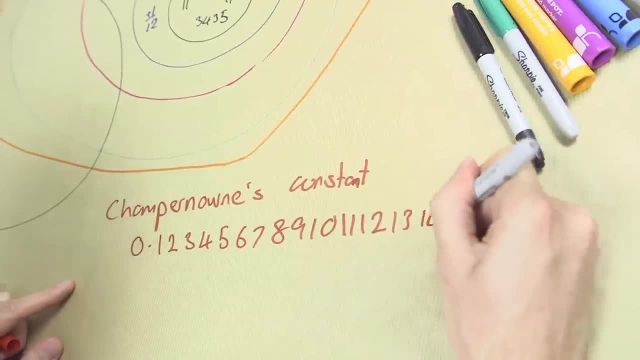 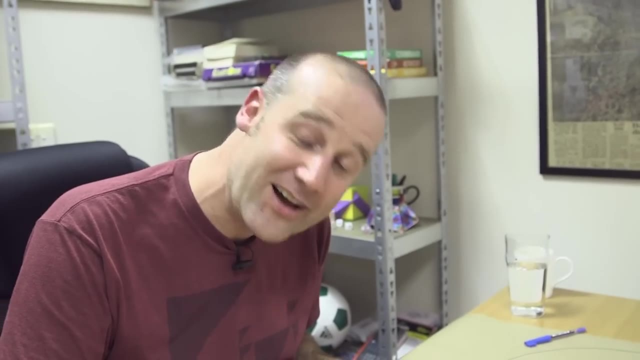 And it's just all the whole numbers: 14,, 15,, 16, and so on: 1, 8,, 1, 9,, 2, 0.. I've got them all And so on. That's like brute forcing the problem, isn't it? 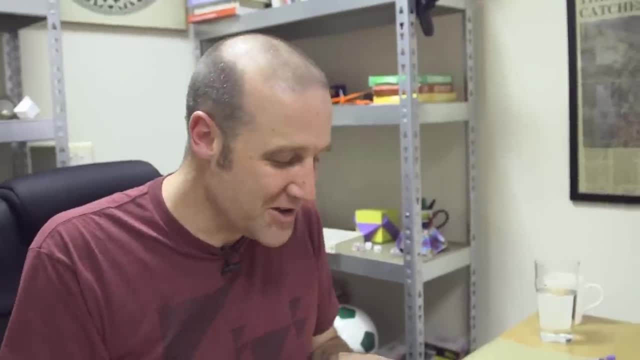 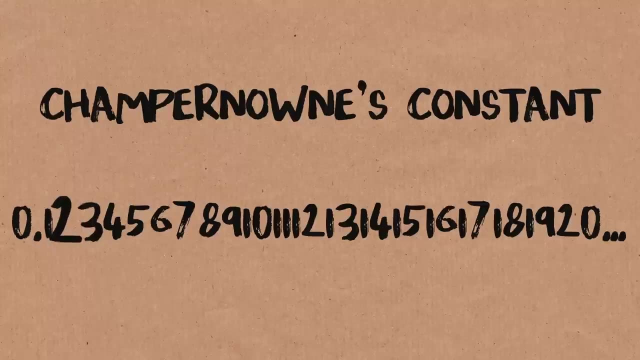 It really is. It really is. I call this an artificial number Because champ noun just went- can I find a number which is normal? And he came up with this procedure. He just went right. You just put all the numbers in order. 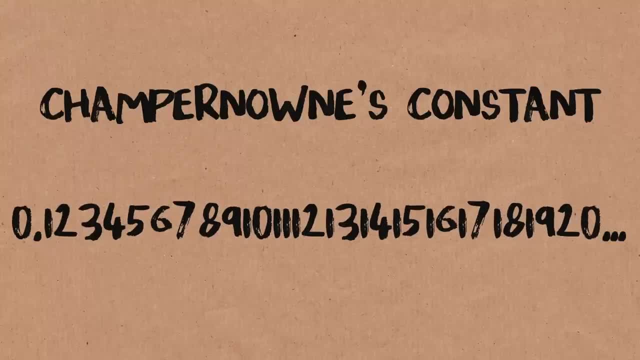 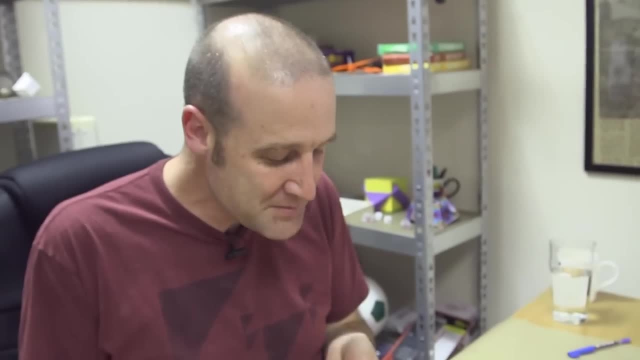 all the integers in base 10.. And you're done. And it's true, Right, Because whatever you want to find, it's in there eventually, Because it's just all the whole numbers listed in there, All numbers listed out And then turned into digits. 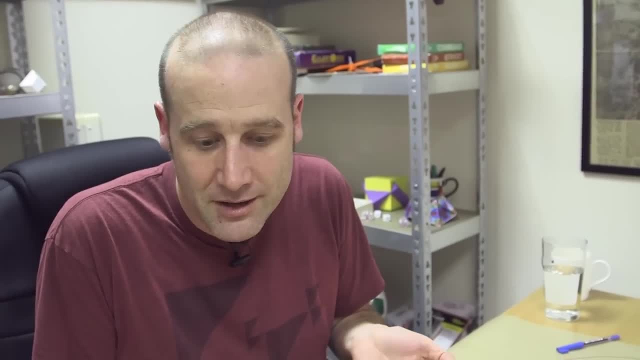 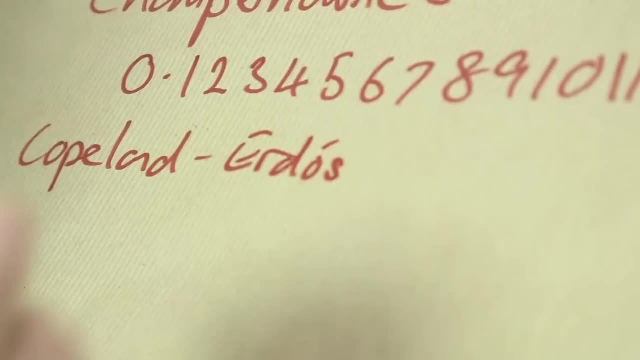 But that's all. numbers are Right, A whole bunch of digits Perfectly valid number Right And it is computable Right. So actually It's like the least efficient way of doing it It is. There's a slightly more efficient one. 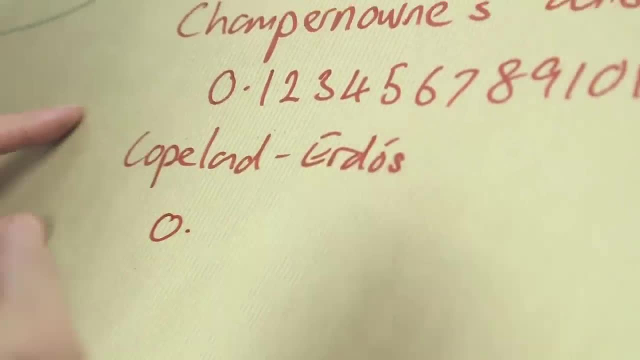 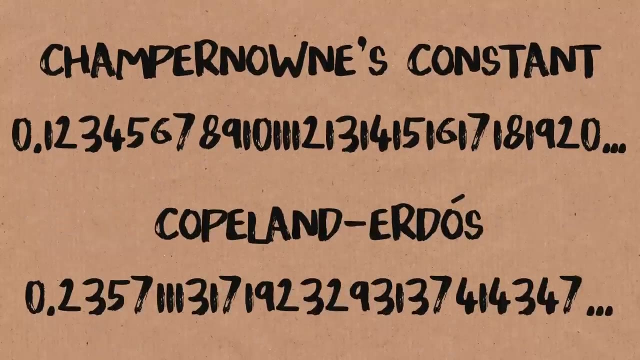 The Copeland-Erdish number is the same idea, but only the prime. So it's 2, 3, 5, 7, 1, 1, 1, 3, so on 1, 7, etc. 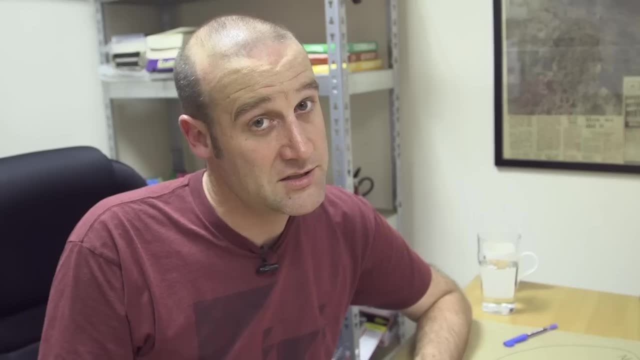 Right, So exactly the same idea, Slightly more efficient. And it's also normal. They didn't start with these numbers and go. I wonder if they're normal. These people sat down and went. I'm going to make a normal number. 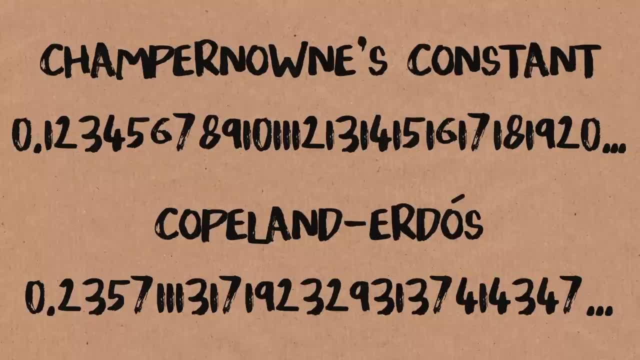 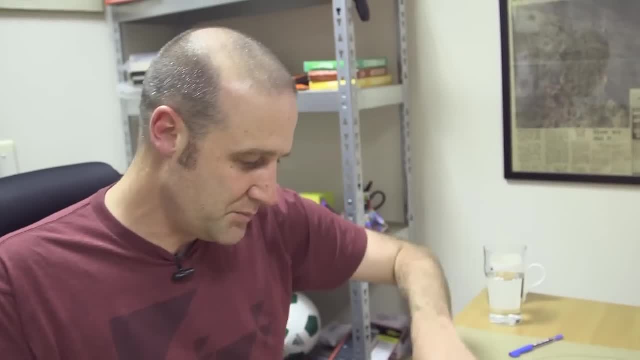 How can I do that? And they generated these. Now, Champagnon's number is transcendental, So this is it in base 10.. Obviously, you can do it in different bases, And it is computable, It is normal And it is transcendental. 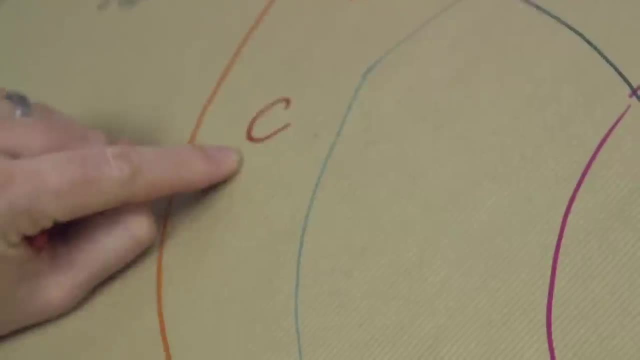 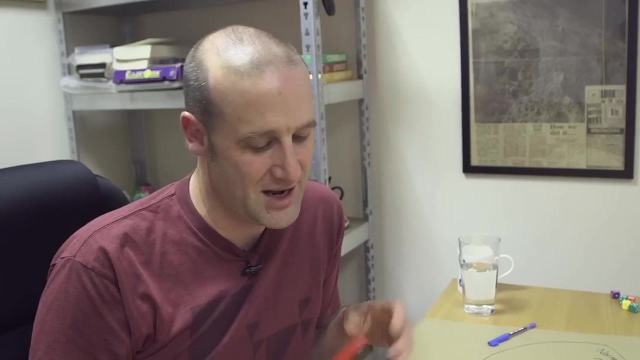 So transcendental means it's outside, algebraic: It's there And not the speed of light. Champagnon's constant sits in this part of the diagram, So the only normal numbers we know for this number are artificial ones that have been constructed for that purpose. 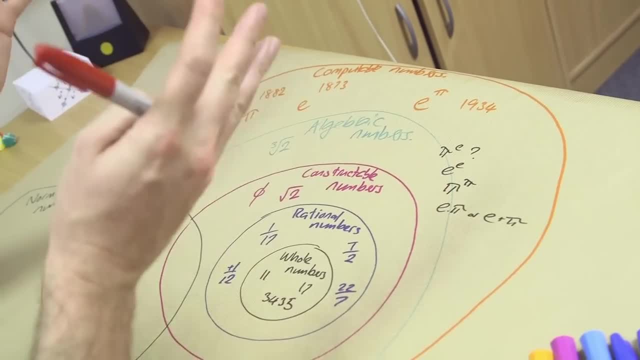 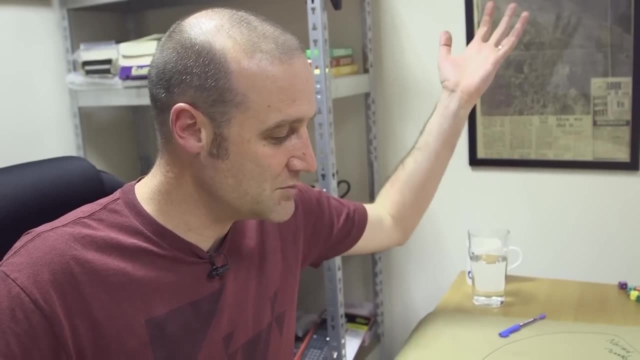 We have never started with a number and then discovered it is normal. We have no test. There is no process for taking a number and proving it's normal Mathematics. hopefully one day we'll have a test. Currently we don't, Which means all the normal numbers we have. 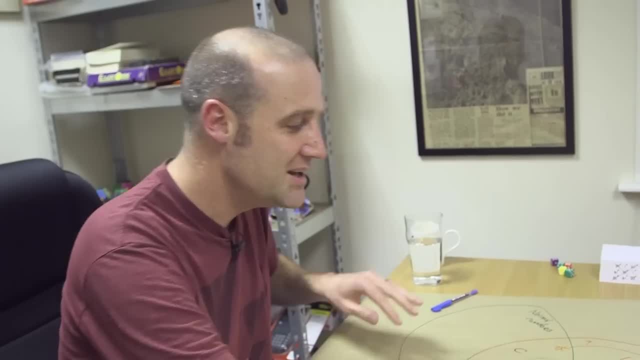 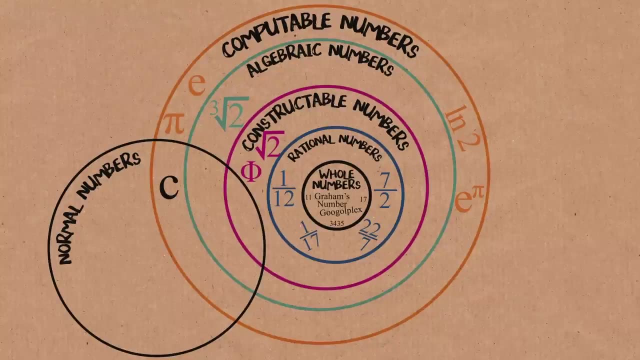 are artificially generated. We are yet to take anything from here and show that it's allowed to move over this line. There's an elephant on your diagram there. Is it over here? Yeah, Well, very interesting. you should say that, Brady. 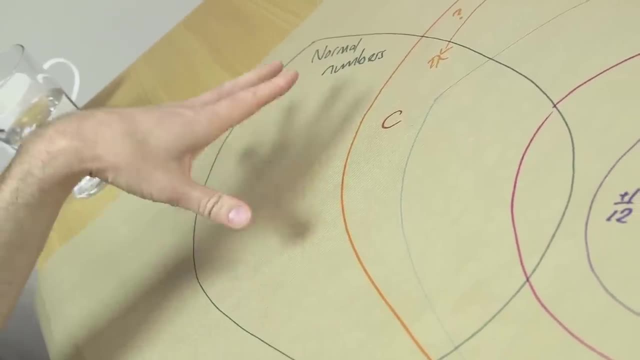 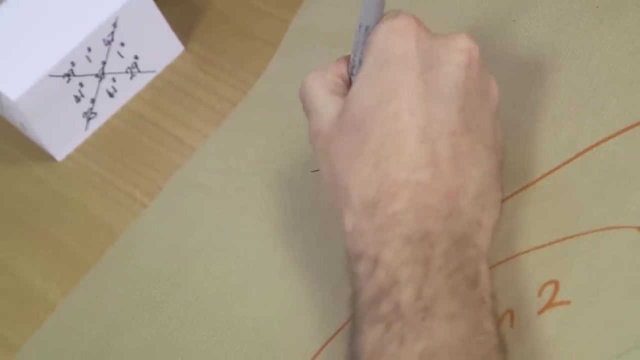 This section is empty, And this is the only properly empty section of the diagram. Now up here we had that one number whose name I couldn't remember properly: Chiton, Or this set of numbers due to whether or not a program will halt. 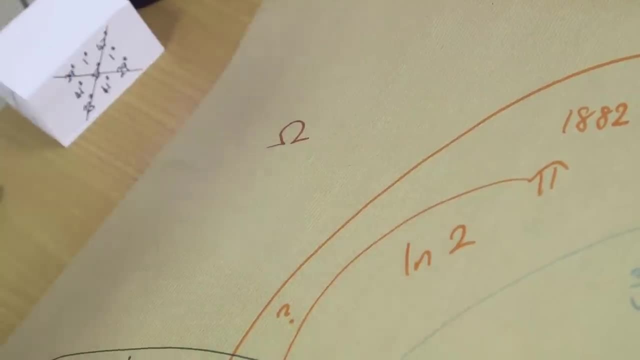 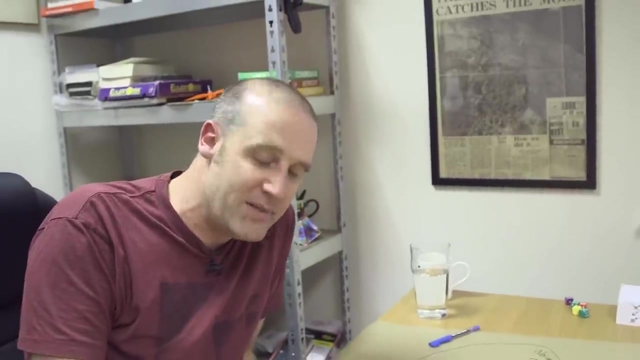 We've got numbers in this category, right? So this section, we've got numbers. This is completely empty, And that's because the only normal numbers we know of are ones that we made for that purpose And the fact that we made them for that purpose. 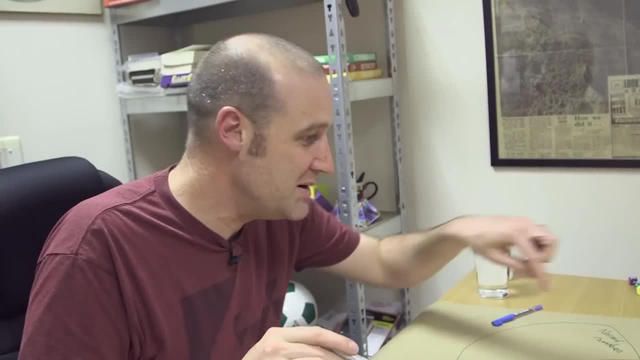 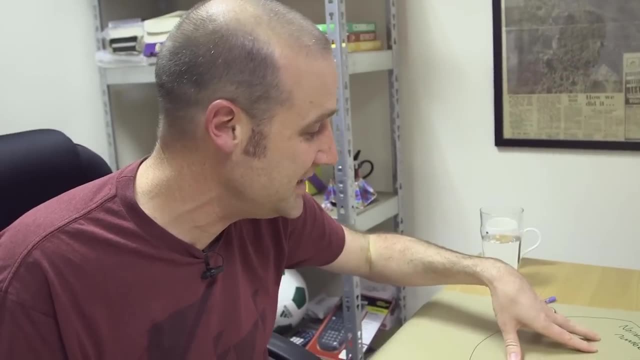 means we have a rule for generating them, which means they must be computable. To have an uncomputable normal number would be incredible, But this is currently empty. But we have managed to prove one thing: We've managed to prove that most numbers are normal. 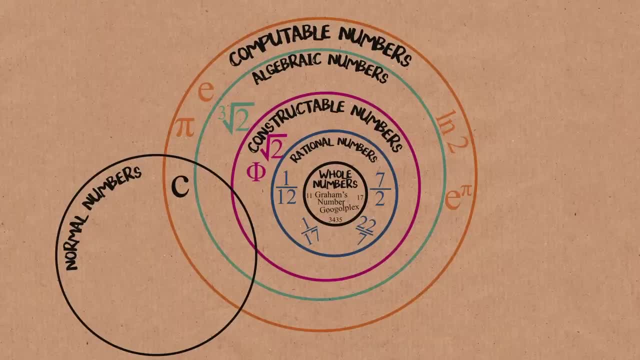 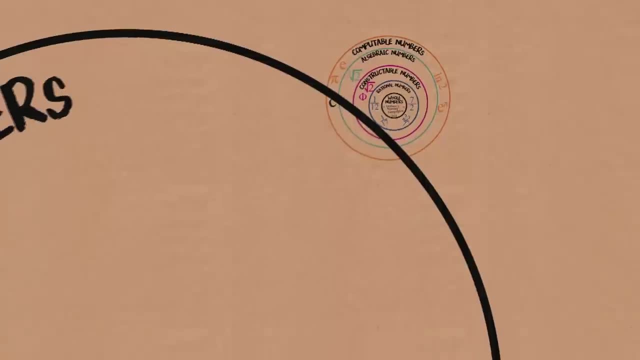 And most numbers are uncomputable. So actually this is the biggest section. This is numbers right. This is a trivial blip right In the world of numbers. This is where numbers are Right And we have none.